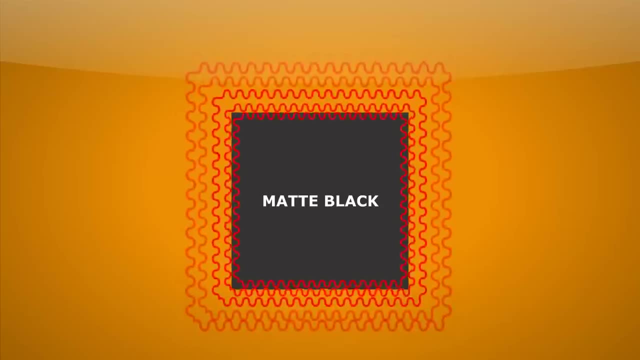 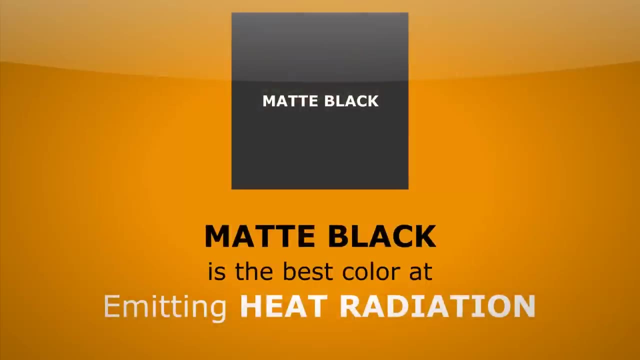 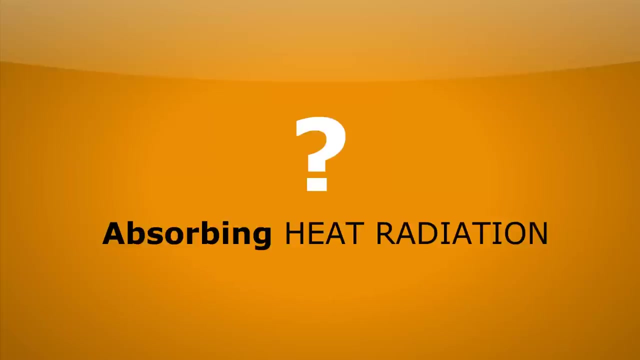 see the matte black side. we can see that is going like crazy. That is emitting loads of heat radiation And we can see from this that matte black is the best colour at emitting heat radiation. So what colour is going to be best at absorbing heat radiation? We've seen that- matte black. 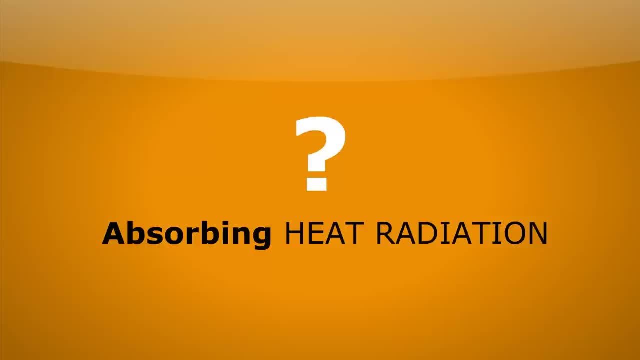 is definitely the best emitter, but what colour is going to be the best absorber? So there's a really easy experiment for this. We have a nice heat source in this form of a fire and we can stick, using just some wax, two marbles onto a couple of plates- One plate. 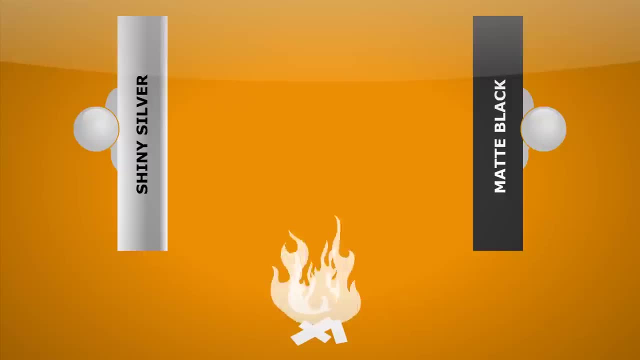 with a shiny surface and one plate with a matte black surface. So whichever surface absorbs the most heat radiation is going to melt the wax the fastest and therefore the marble will drop quickest. So which one do you think it will be? Well, let's look. and 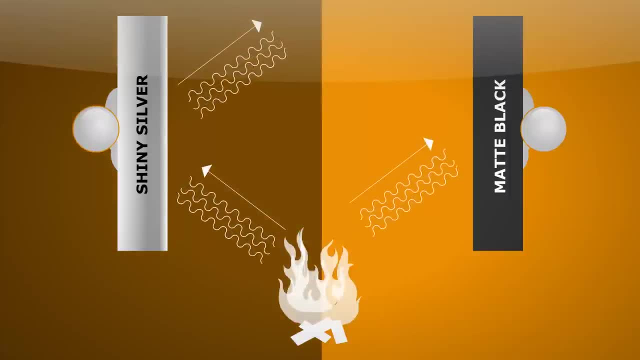 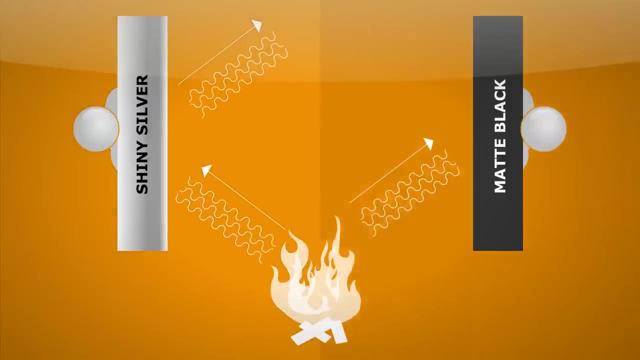 see what happens. Well, first off, I can notice that the shiny silvery surface is reflecting away all of the radiation. The matte black surface seems to be absorbing all that radiation. So I'm going on the. oh, there we go. The matte black fell off way in advance of the shiny silvery. 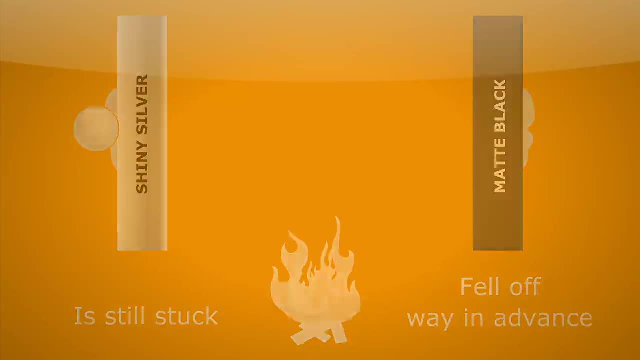 one, The shiny silvery one, is still pretty stuck on there, And we can see why It's: because matte black is absorbing all that radiation. shiny silvery is reflecting it. So what's the key information for us to have here? Well, when heat needs to transfer across, 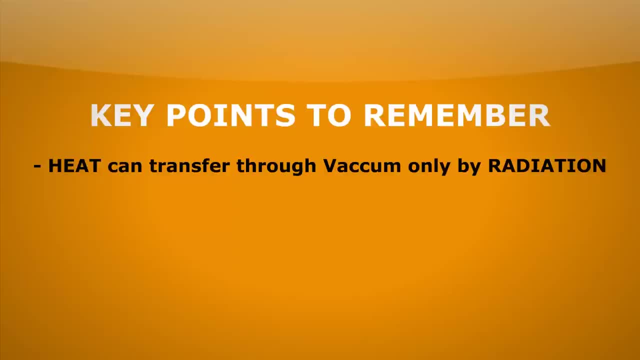 a vacuum. the only way it can do it is by radiation. We've also seen that matte black is the best absorber and emitter of radiation, And that's why, if we want something to heat up really, really quickly or something to cool down really, really quickly, we colour it matte black. 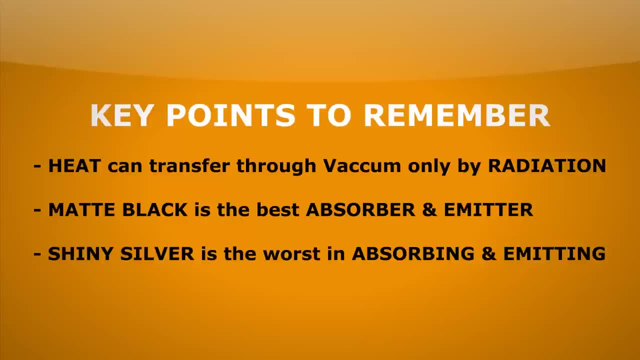 We also saw that shiny, silvery surfaces were the worst at both absorbing and emitting radiation, and that's why, if we want something to stay hot or if we want something to stay cold, use a shiny, silvery surface.